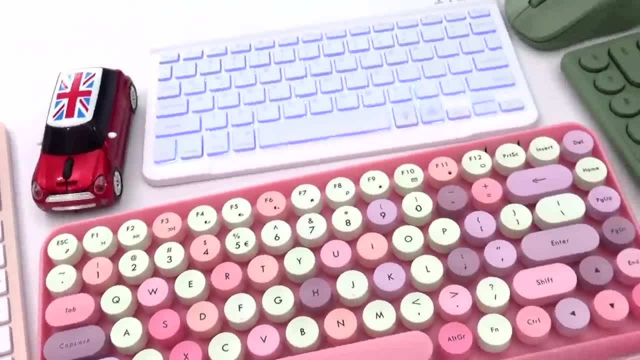 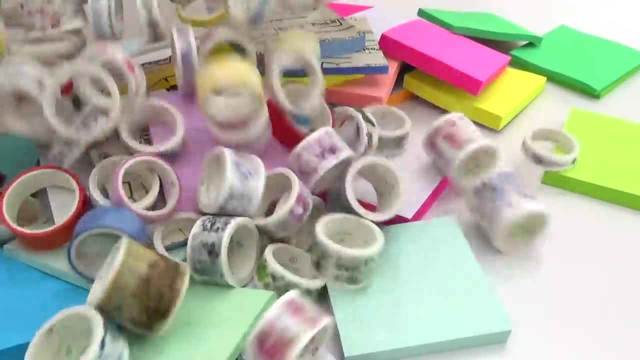 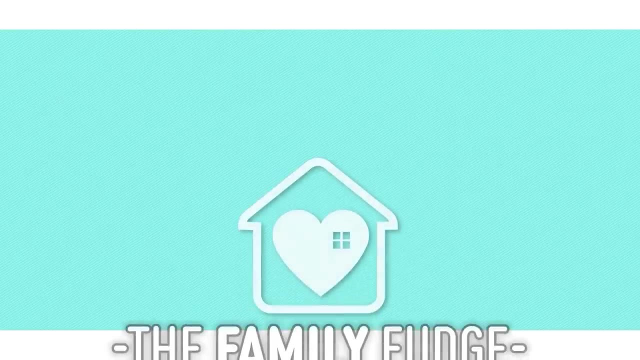 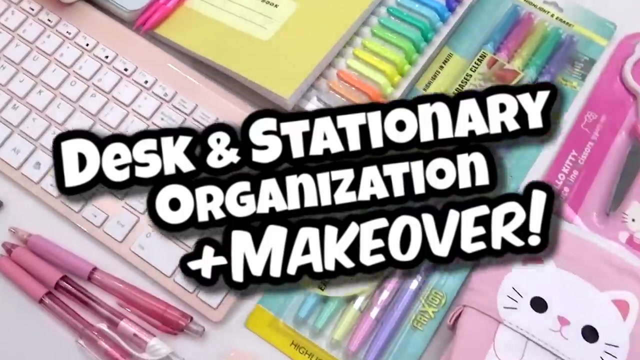 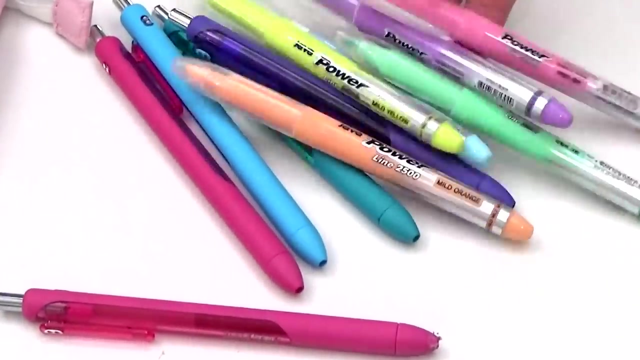 Hey everyone, Jennifer here, Welcome to the Family Fudge and welcome to part two of our back to school series. In last week's video, I shared with you our huge back to school haul, But in today's video I'm super excited because I'm going to be taking you along with 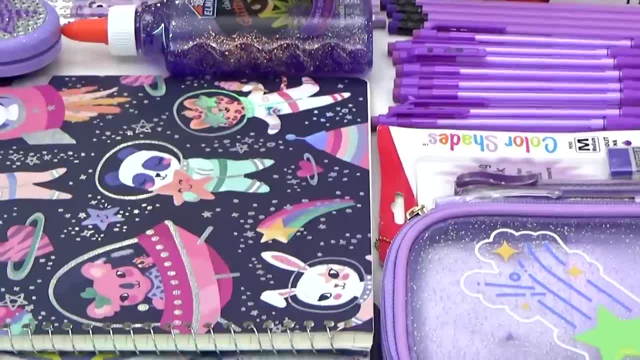 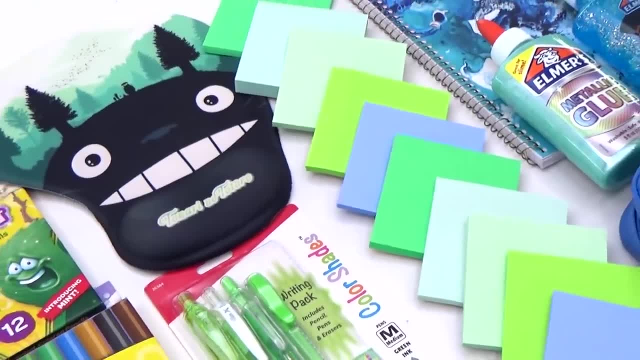 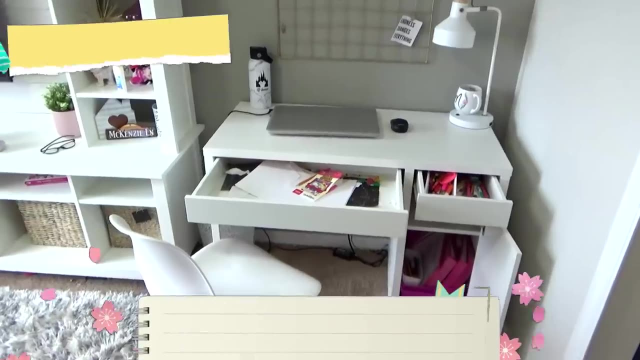 me as I give each of my kids desk area a makeover. Now, before we get started, don't forget to give this video a big thumbs up if you love school supplies and organization, And don't forget to hit that red subscribe button if you haven't already. Now for these desk spaces. 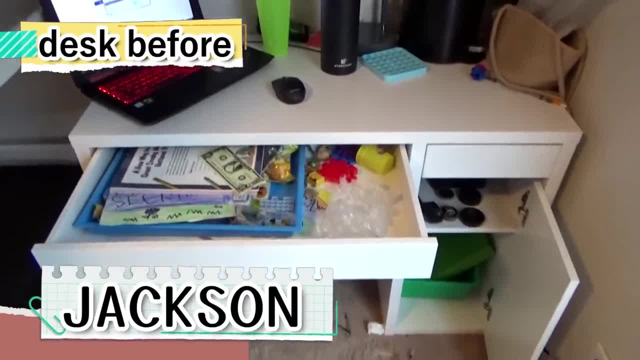 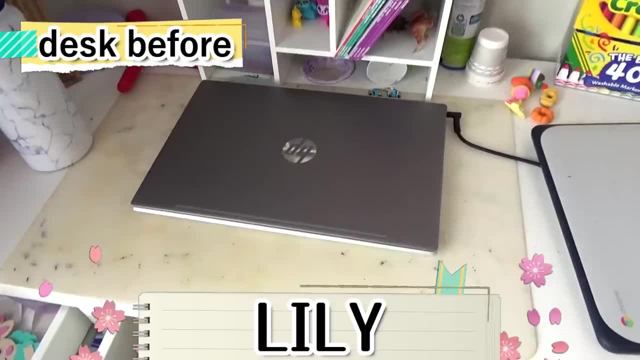 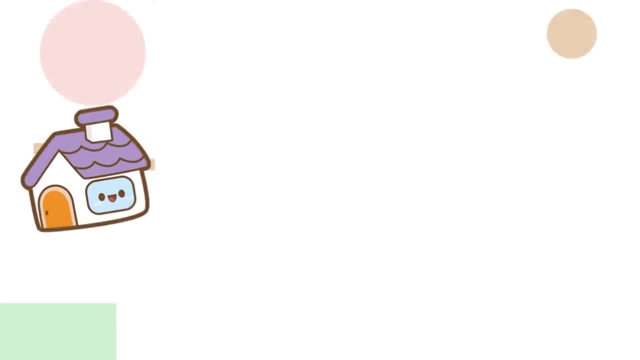 it's really my goal to create fun but functional spaces. I want these areas to be cozy and comfortable for my kids. I think that's going to make studying time a lot more enjoyable, And I also want each of my kids desk areas to kind of reflect their personality. Before I can start, 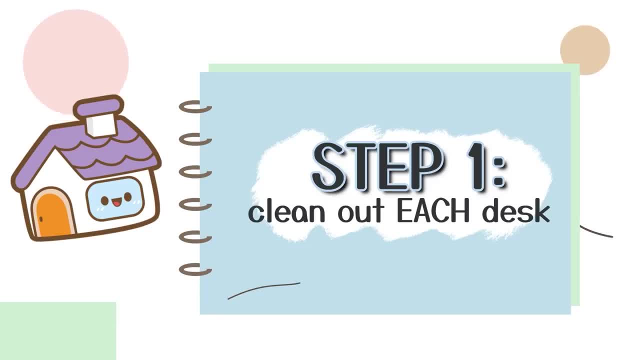 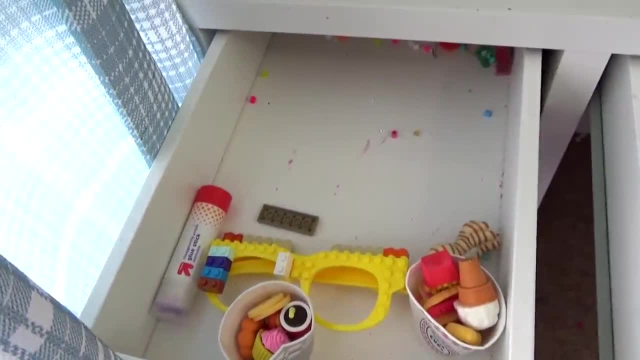 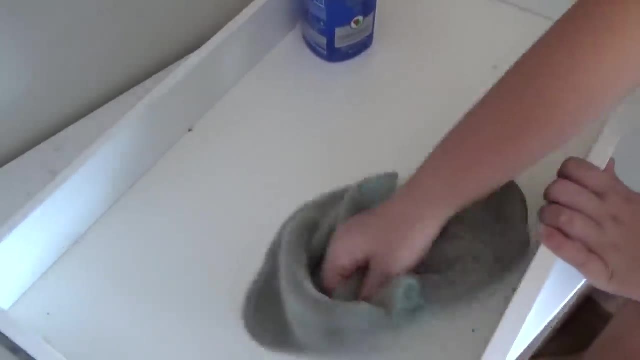 bringing in all of the new school supplies. we're going to need to take out and go through all the stuff from last year. First, we're going to take everything off of the top. We're going to take everything out of all of the drawers. Next, we have some cleaning to do. I'm not quite sure how. 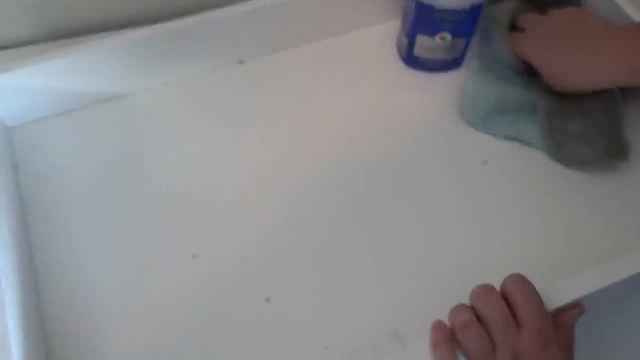 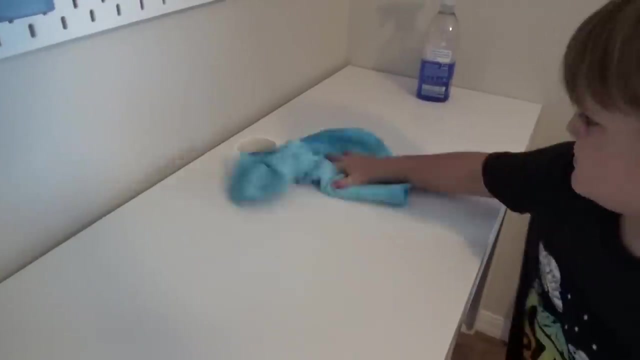 the inside of the doors get so cruddy, but they definitely are, So we're going to wipe them out. We're also going to wipe down the tops of each of the desks as best as we can, And then, finally, we're also going to need to do quite a lot of vacuuming. 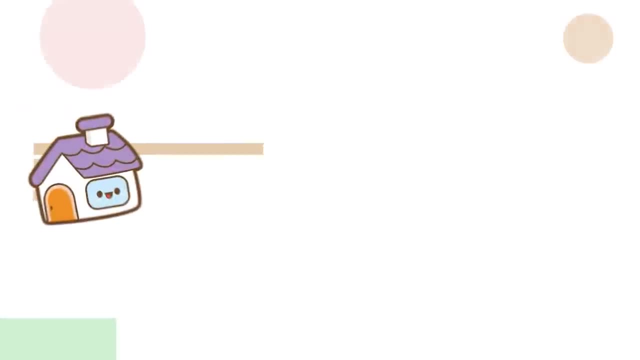 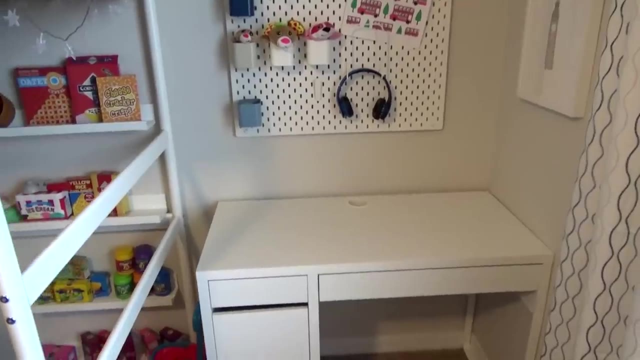 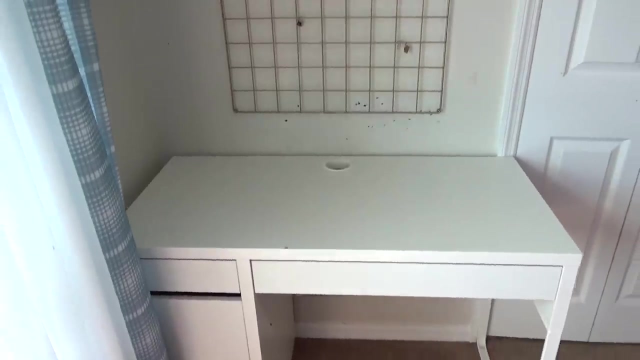 So, now that I essentially have four blank slates, I'm going to go ahead and take over. I'm going to go ahead and set up everything for my kids, because that's kind of my favorite part. I love getting everything organized, And then they're going to see the final product I am going to be making. 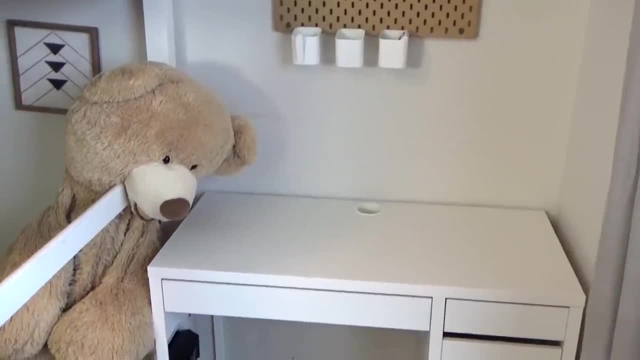 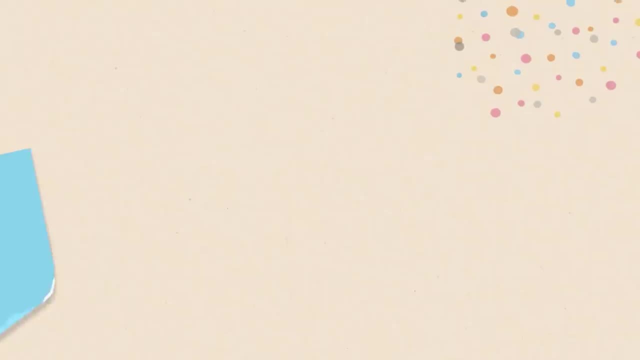 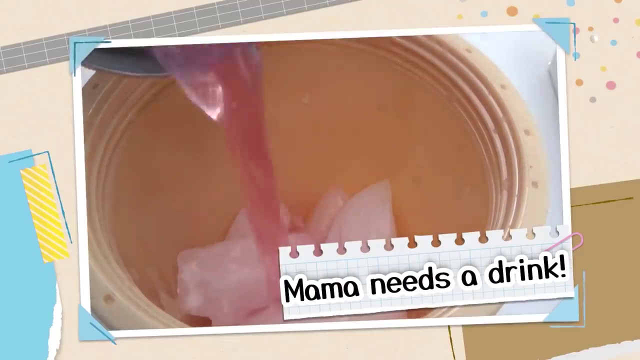 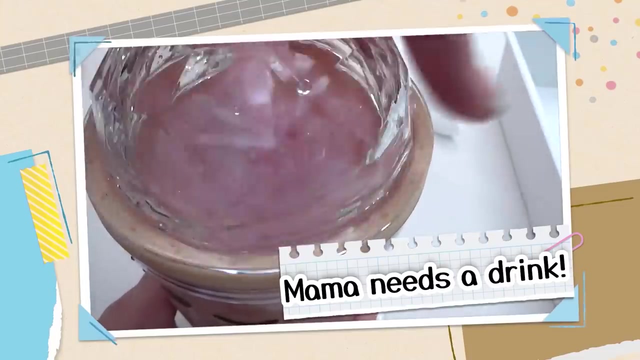 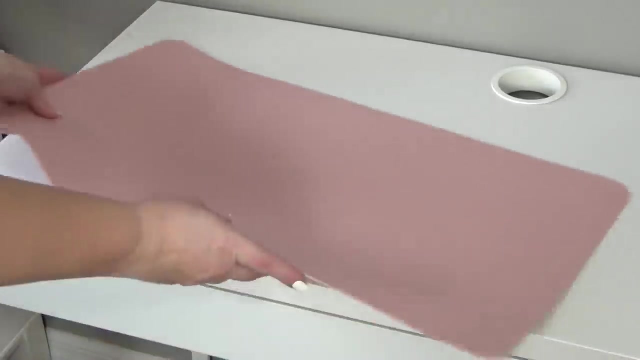 over four different desks today, but I'm just going to work on one desk at a time, starting with Mackenzie's desk. But as I'm working, I do need a drink. The first thing I'm going to add to Mackenzie's desk is this really pretty desk protector Now? 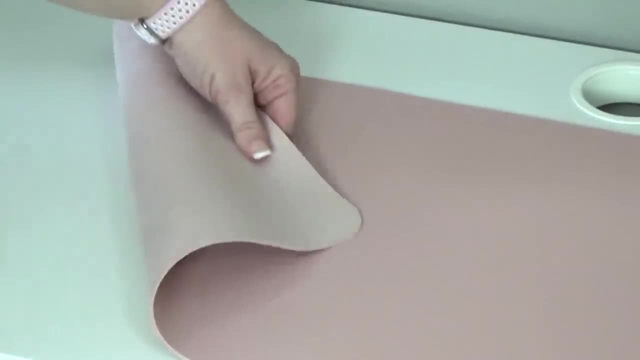 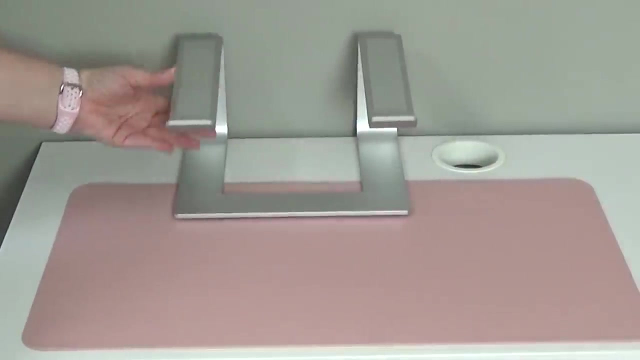 this is something I didn't have in last week's haul, but I did end up getting one for each of my kids, So I'm just going to go ahead and do that, And then I'm just going to go ahead and set up my kids, because I really want to protect these desks. Right on top of here, I'm adding the. 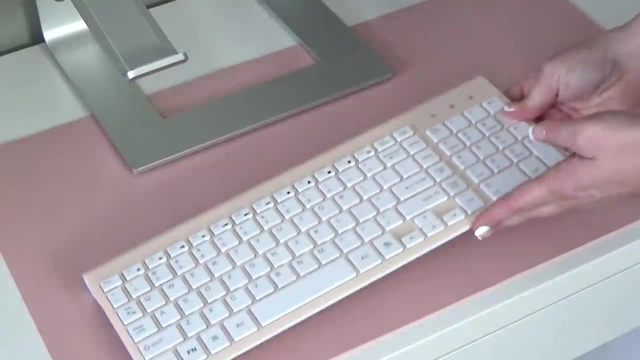 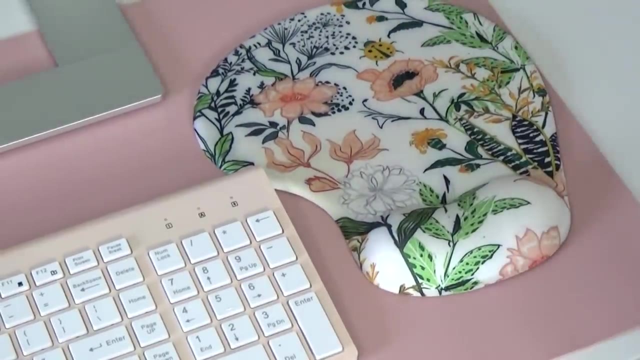 computer stand. My kids all have a couple of online classes this year, so they use computers. They also use tablets, And especially when using a tablet, these computer stands are awesome. It brings them up a little bit higher so they don't have to strain their neck if they're sitting there. 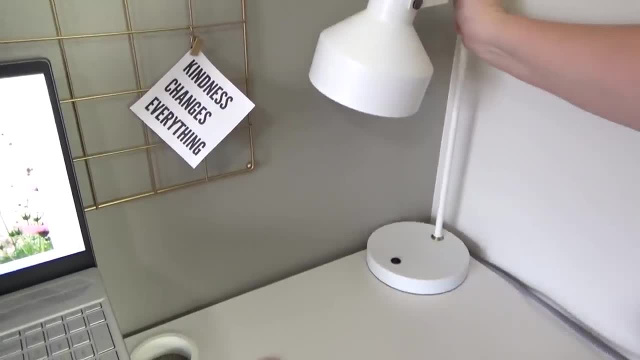 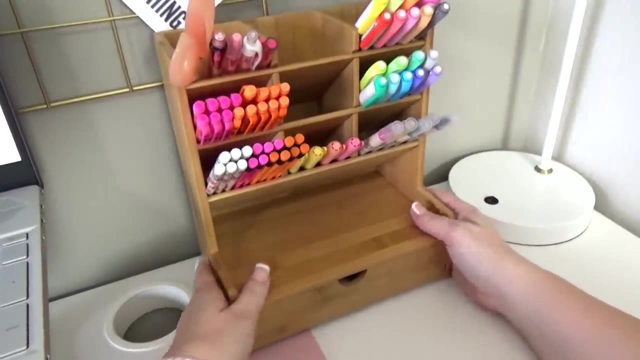 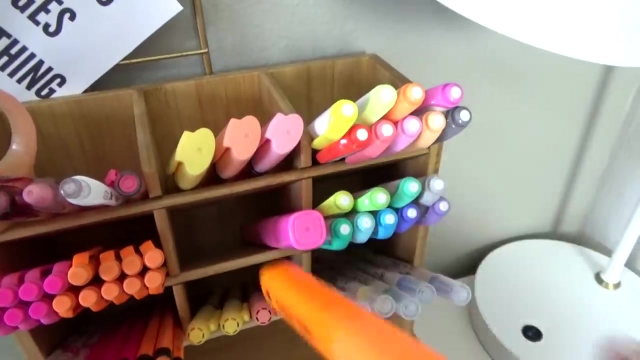 for a while. So it's not going to be an over-the-counter thing, but just the fact that you're going to be using an lunch box or a marker and you can just go ahead and cheat and use that as well. So I'm going to take this one of these and add it to the desk. 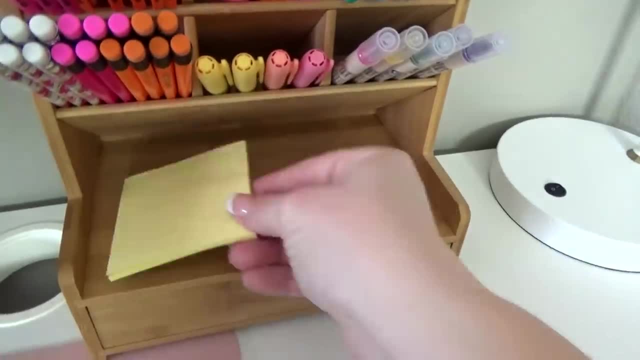 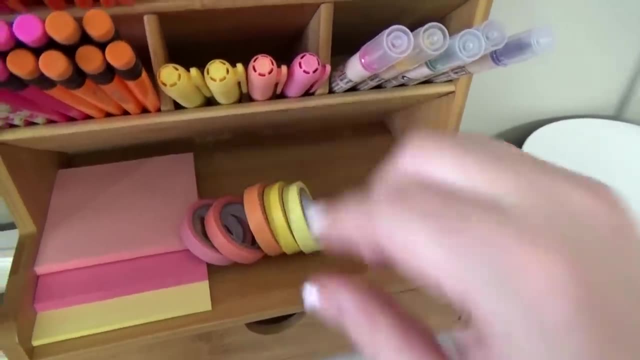 And then I'm just going to go ahead and create a desk for my kids. These are two of the things that you'll be using to decorate your desk. So these are some of my favorite items. I have two sets that I've added to my desk. 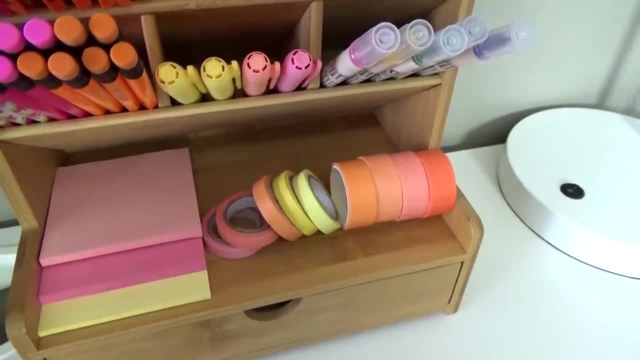 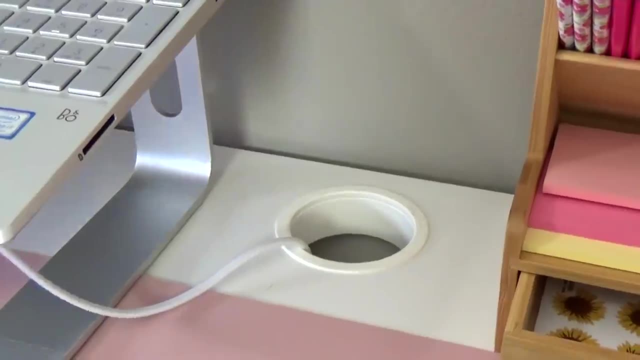 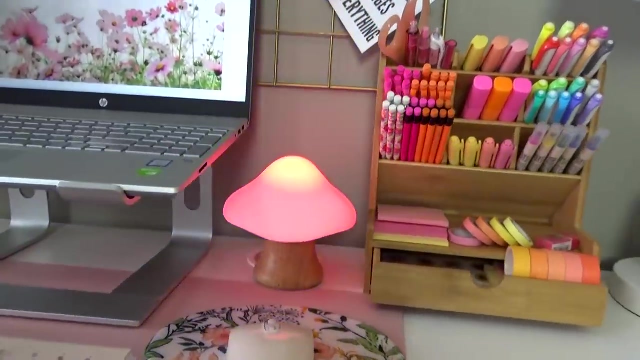 I've added these to my desk. One of them is called a black readers, One is called a silver heures, The other one is called all the others, So they're two different things. Okay, Because this isn't the biggest desk. 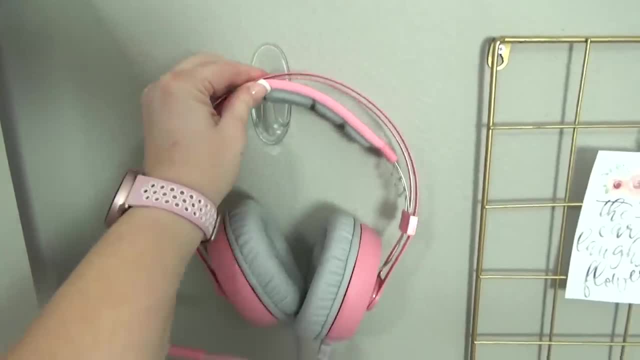 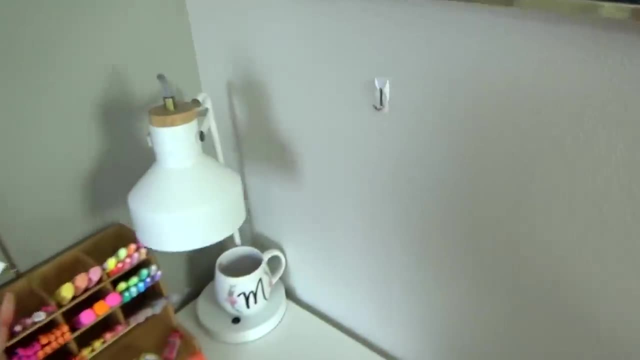 I am gonna go ahead and hang up Kenzie's headphones. I'm just using a command hook to do this. That way, when she's not using these, they can be up and out of the way, And I'm also gonna be adding this clipboard. 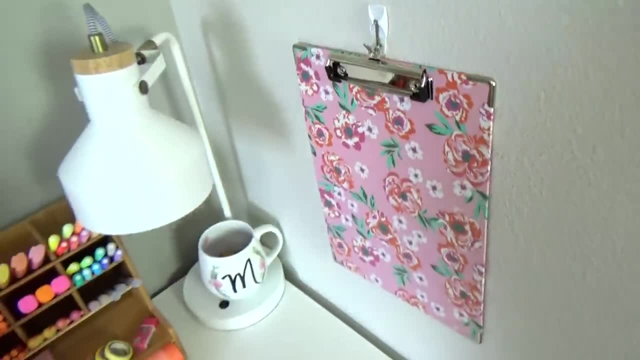 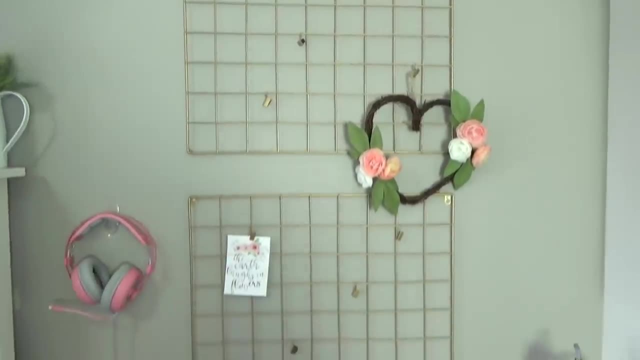 to a command hook as well. This is where McKenzie is going to be hanging up her schedule and her chore list. That way she can see it and hopefully get them all done. Above the desk on the wall, McKenzie has plenty of space to hang up pictures. 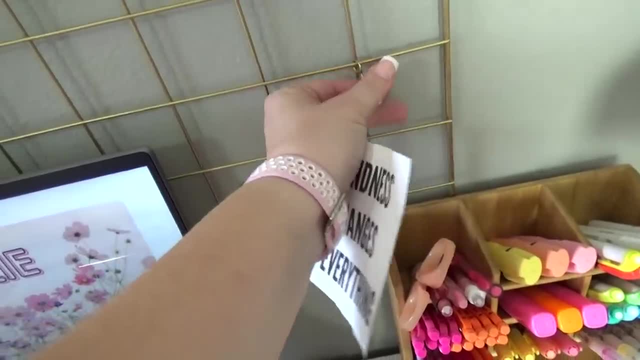 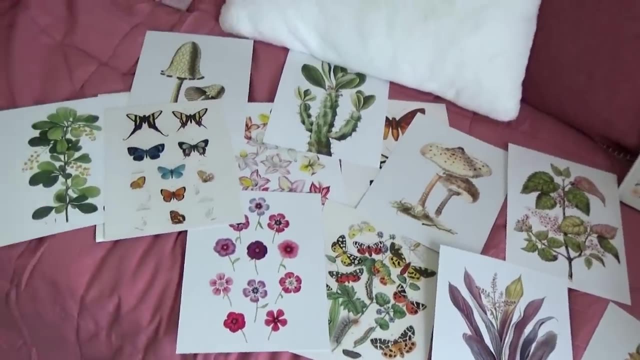 And this is something that she's been wanting to change out for a while. These totally fit her vibe and her style, So she picked out a couple of her favorites and I'm just going to hang them up right here. In this area, I'm also gonna be adding some of this faux ivy. 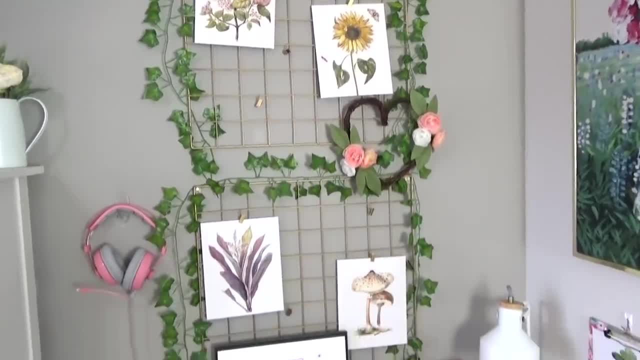 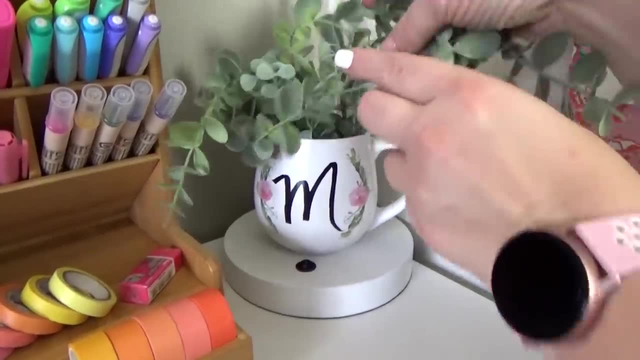 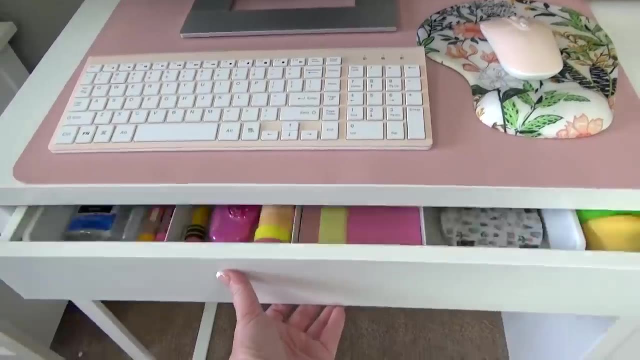 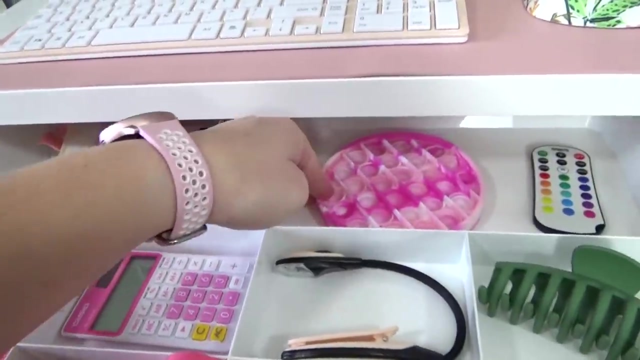 I know this is so trendy right now and I really love the combination of both of these. I think she's going to love it. Moving on to the desk drawers, Instead of using a lot of little containers to organize all of the items, I picked up these drawer organizers. 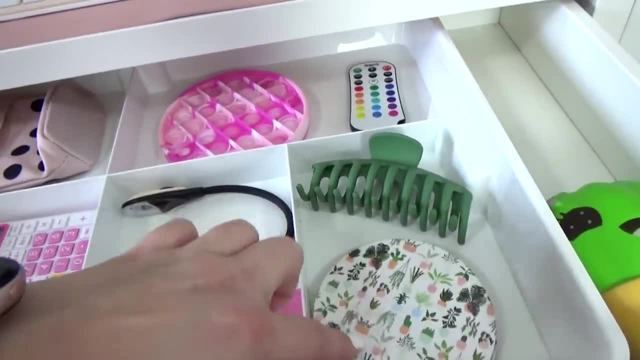 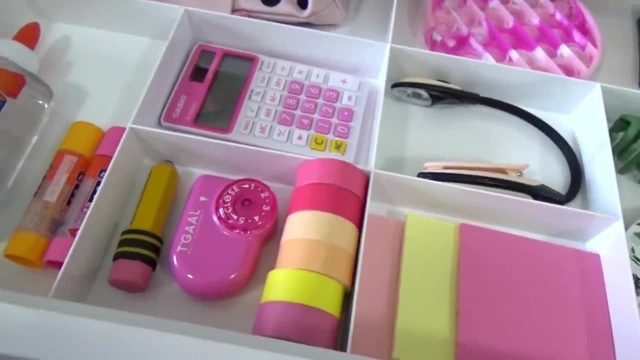 at Ikea. I got one for all of the kids. I also got some for my desk as well. I love that this is one big piece with lots of different compartments to hold lots of different things. Now, most of these things I showed you in our haul video. 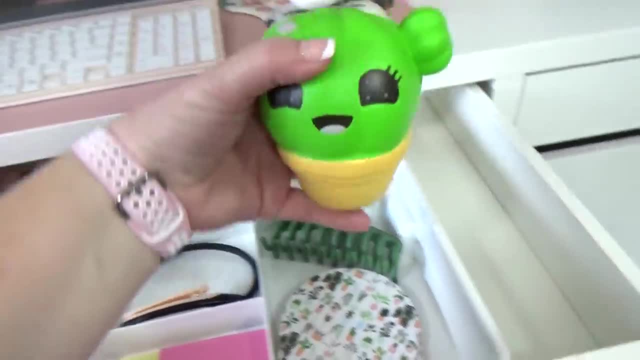 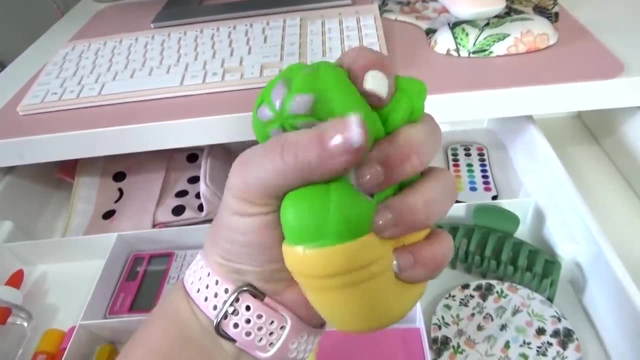 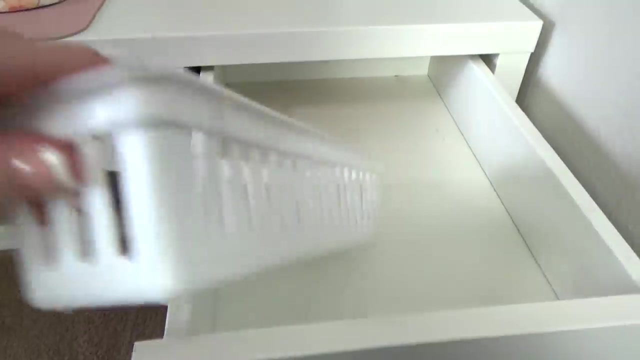 but I did add a couple of extras in here. I added a reading light, a calculator, a poppet and an adorable cactus squishy. Your videos are so much fun to watch. I really hope you enjoy them, Even though I'm in a very good mood. 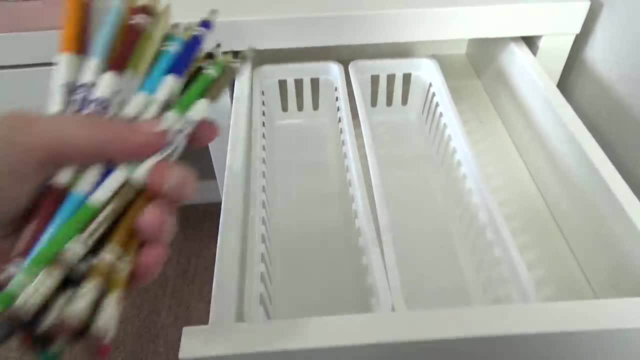 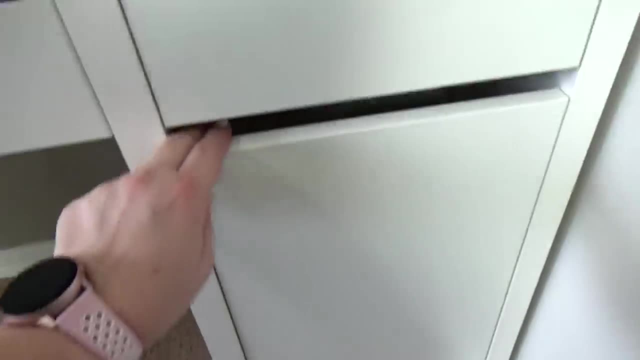 I'm so excited to go home and get back to work. I have to get to work to live. Okay, so I'm ready to go home. I bought a arriving dress. I used to wear a press-on dress throughout my trip. I got it from a Vannity store and I'm back in LA. 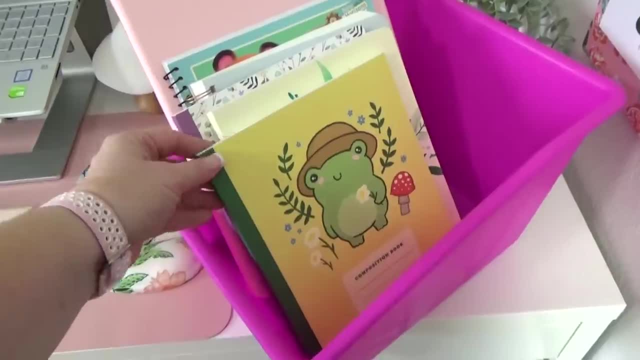 I think I'm going to wear it around the house. It's a little on the back, but I think it's gonna fit just fine. I also picked out a couple of black and white dresses. It's a classic, classic arily blue dress. 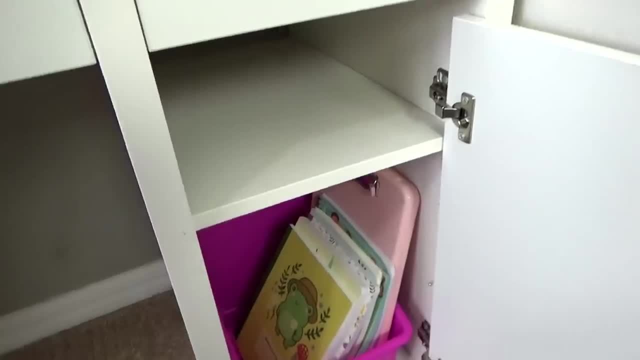 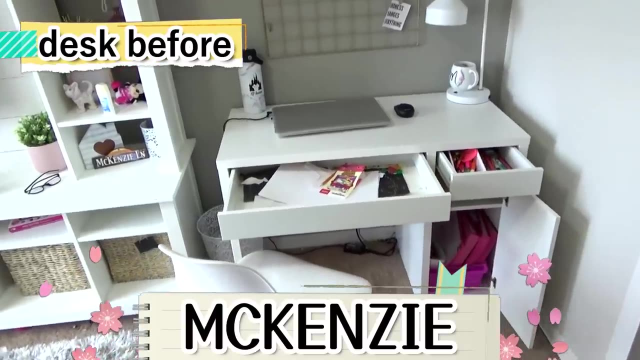 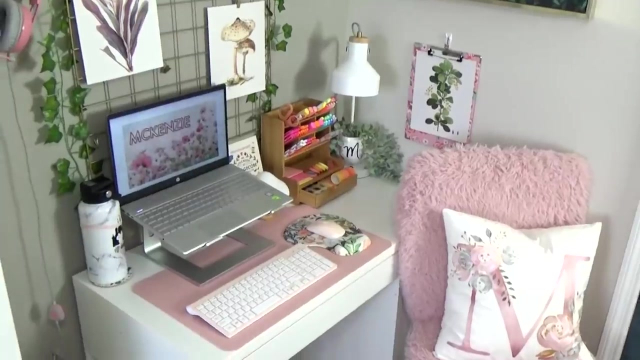 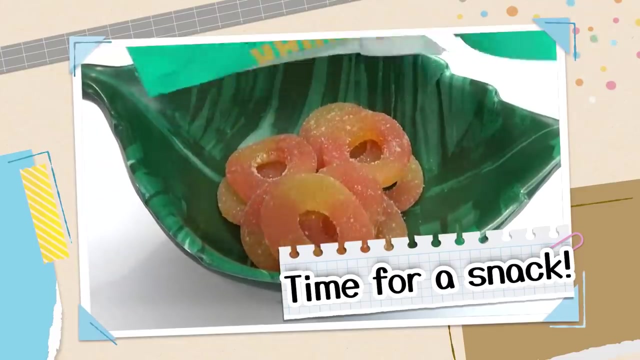 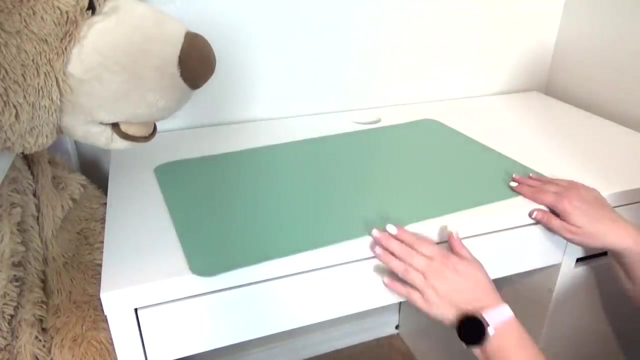 I think I'm just going to go with it. Ah, this one is a little bit too tight. I think I'm going to go with this. It's a really simple dress and, just like that, it's time for a snack for jackson's desk. i'm starting off with that protective mat, just like i got for mckenzie. 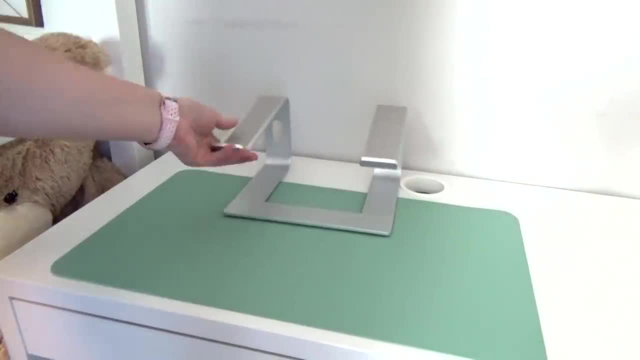 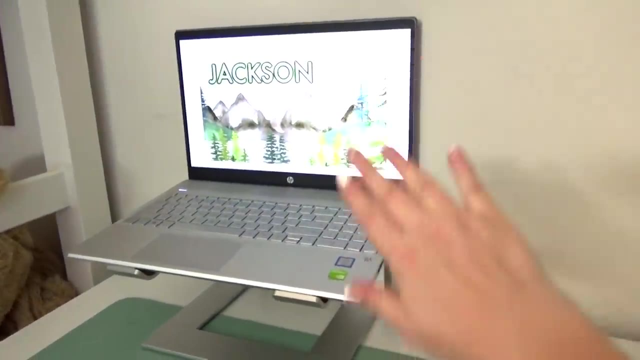 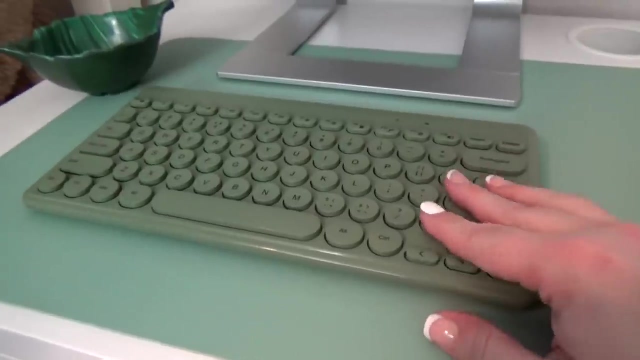 but of course for jackson i went with the green color. this totally matches his room. next, i'm going to add a computer stand. this is going to be perfect for jackson's laptop and you guys, this is also just like mckenzie's. it's the same height and everything, and even though jackson is two years, 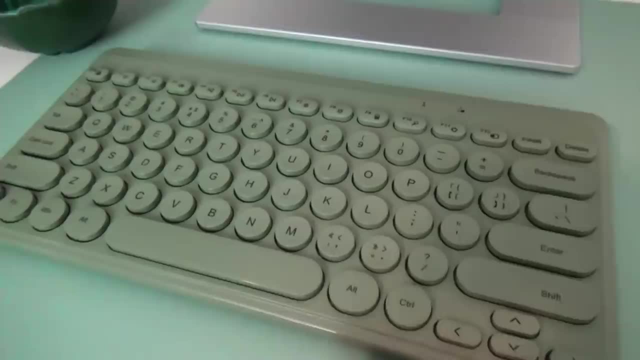 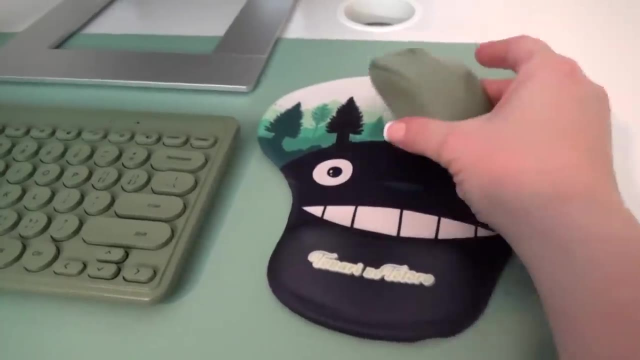 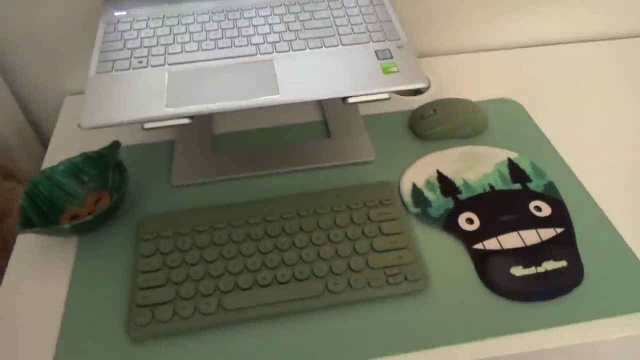 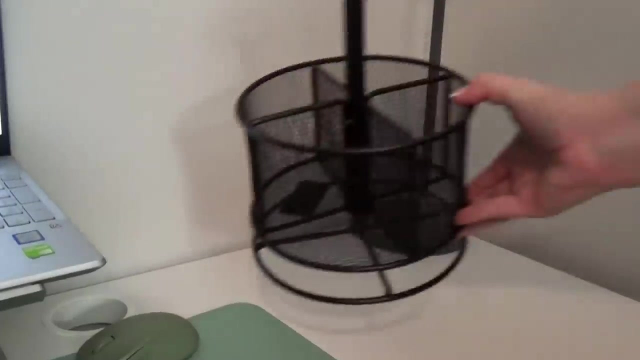 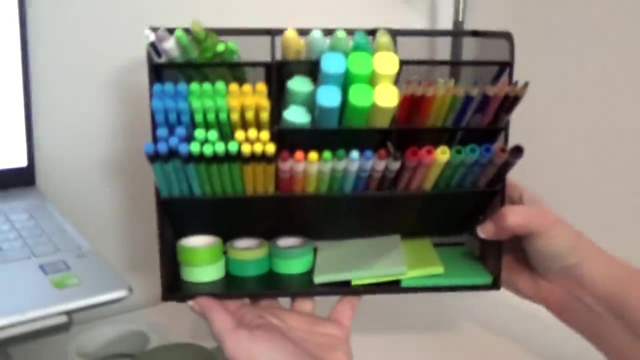 younger than mckenzie. they're almost exactly the same height. in fact. sometimes they kind of look like twins. you now to organize jackson's pencils and pens. i was planning on using this guy right here, but instead i decided to swap it out with this one. this one is a lot like the one mckenzie has. 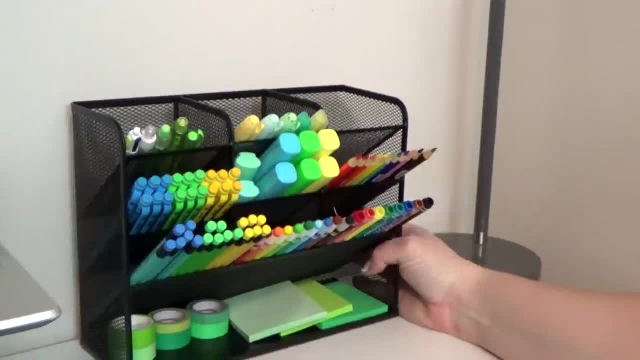 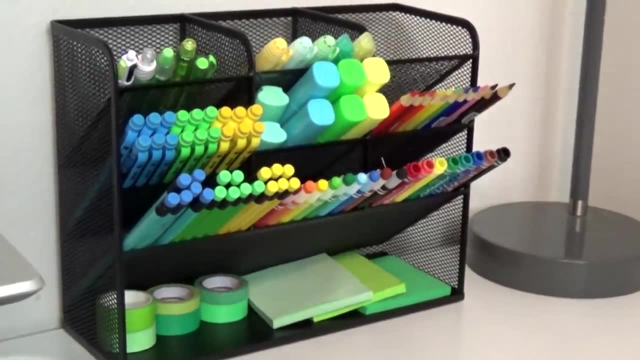 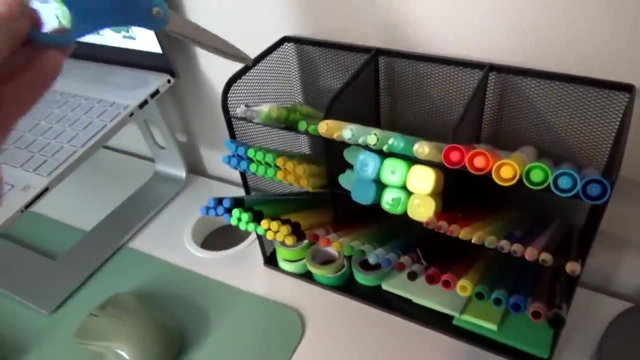 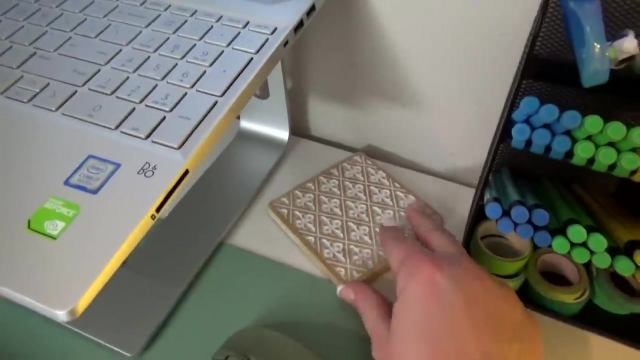 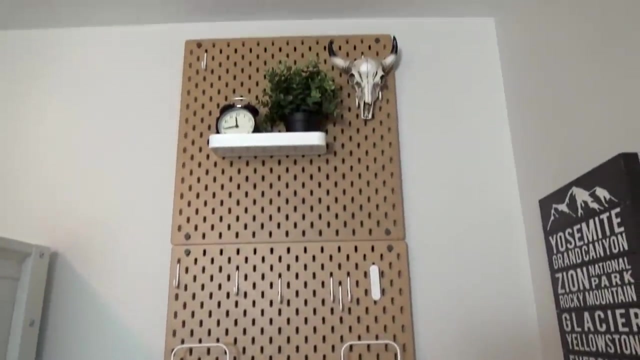 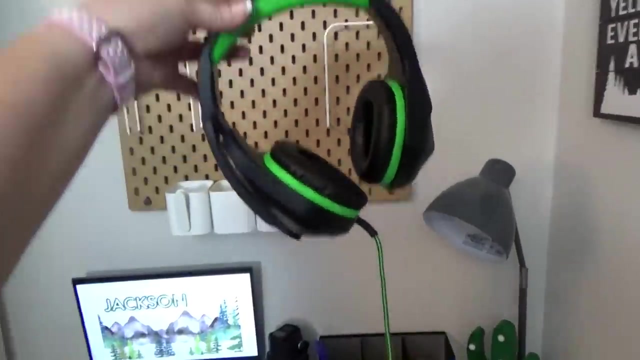 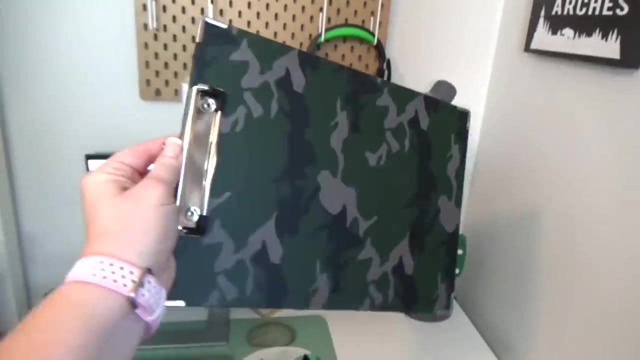 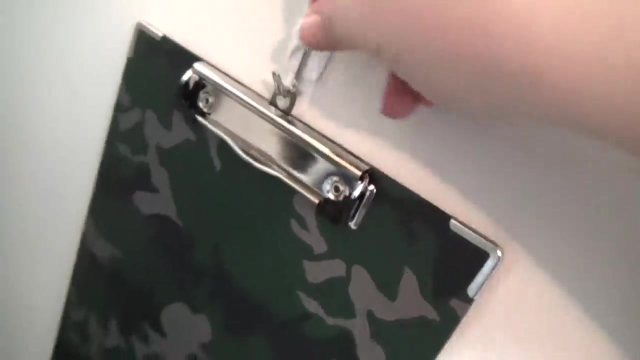 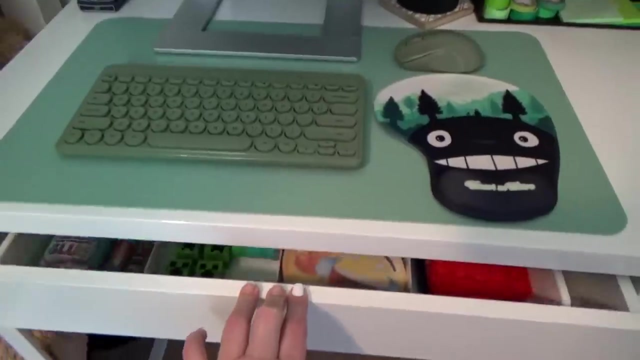 except that hers is wood. i definitely think this one fits better on him. the desk top, and i like that. this one has little compartments to keep everything organized. so now down in the big desk drawer, you'll see, i've added all of jackson's other school. 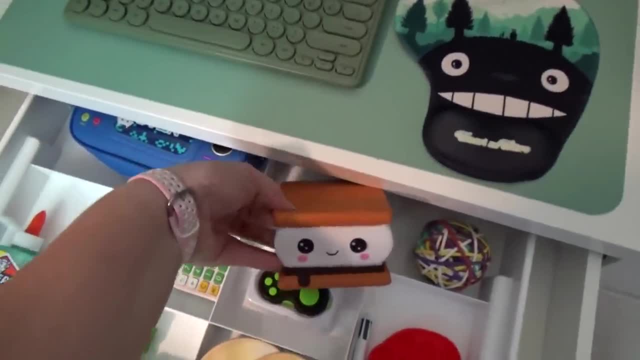 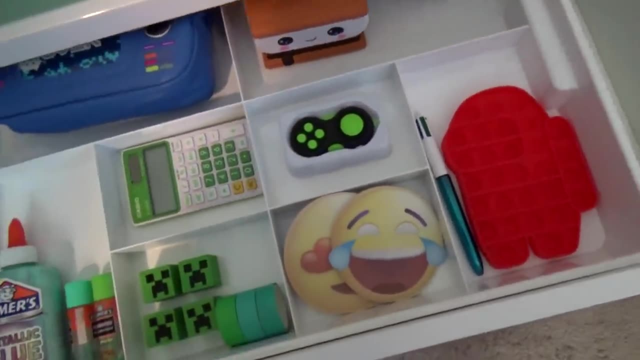 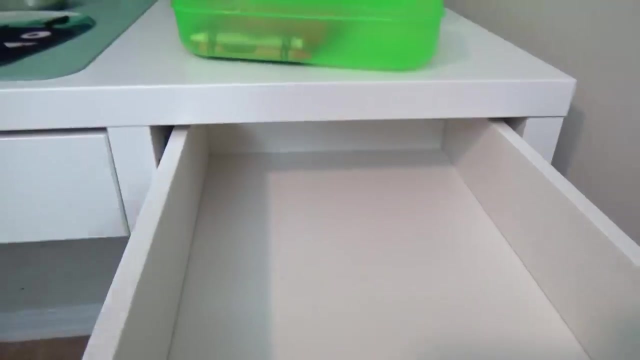 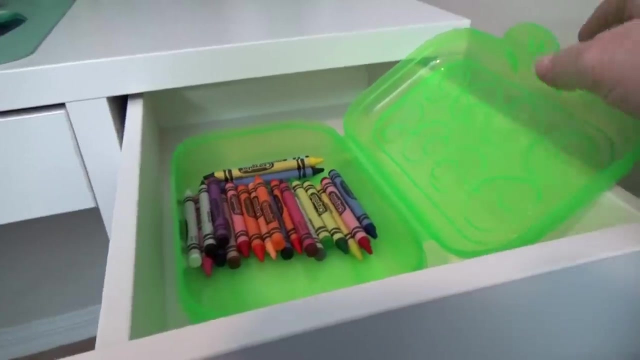 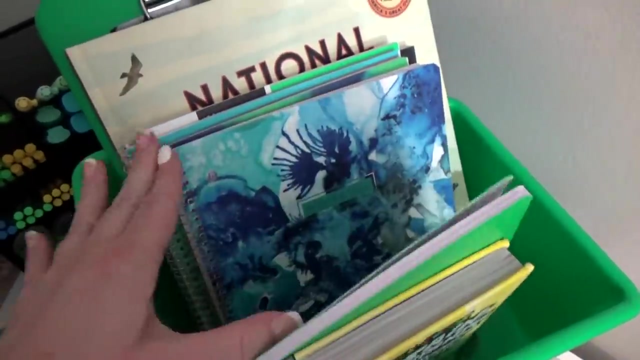 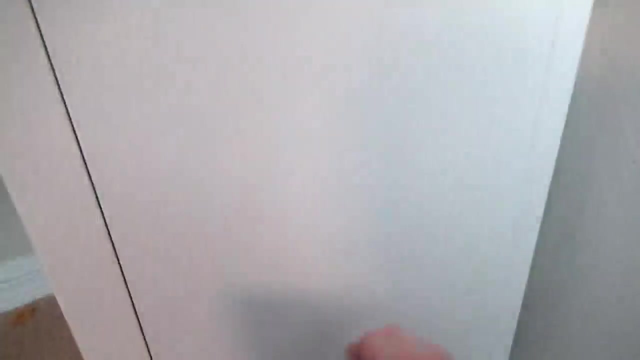 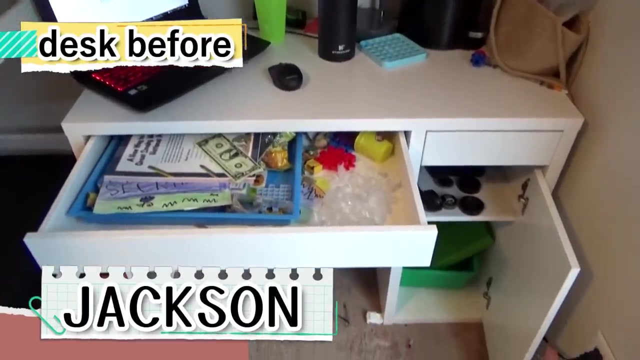 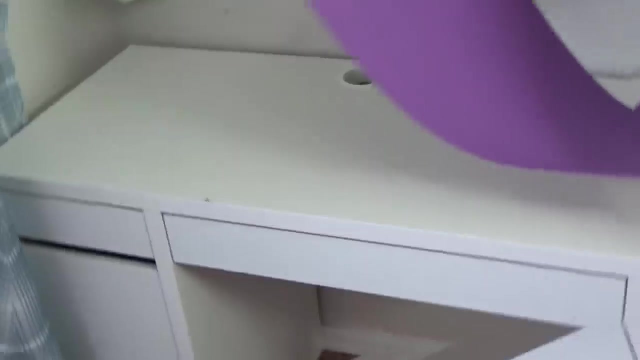 supplies, but i also added him a few extras that i know he's going to love sheet. so on to lily's desk area. for her, i decided to go with a purple desk pad. lily loves all things area for her, i decided to go with a purple desk pad. lily loves all things. 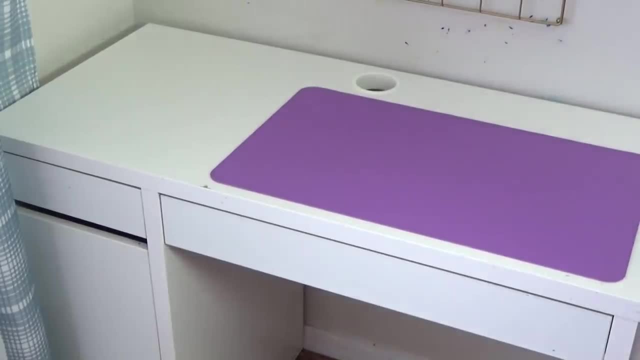 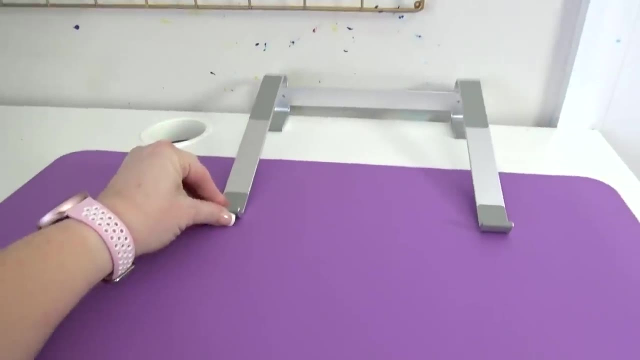 loves all things purple and pink, and she also loves pandas, So you're gonna be seeing a lot of those in this area. Next I'm going to add her computer stand And you guys while I'm working on Lily's desk. 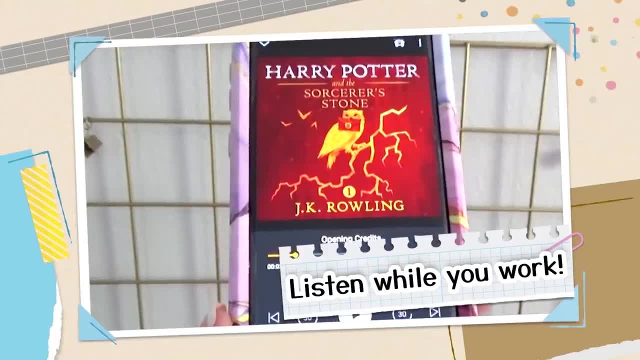 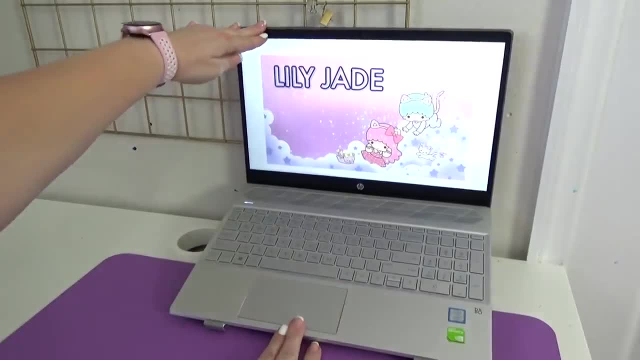 I decided I needed something to listen to. I decided to go with one of my favorite audio books. You guys will have to let me know in the comments down below if you've ever listened or read this book before. So let's get started. 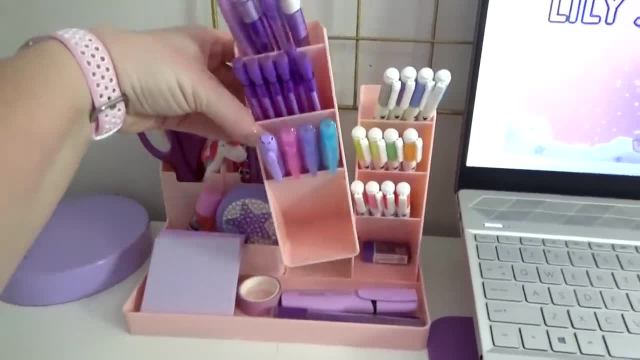 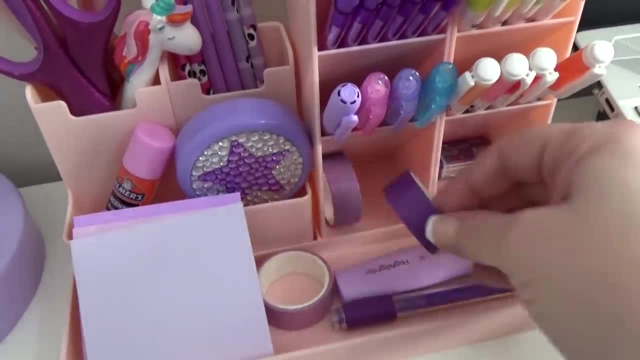 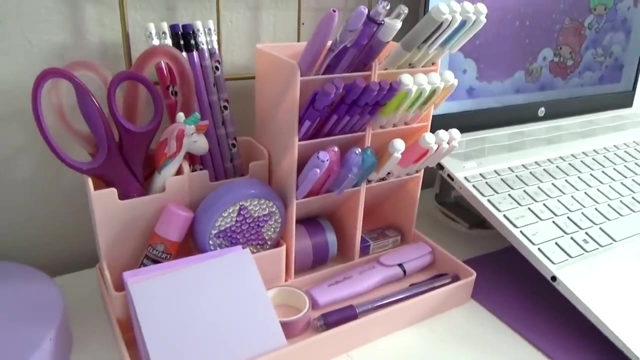 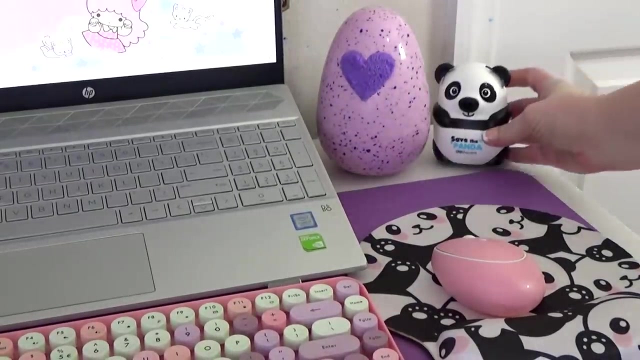 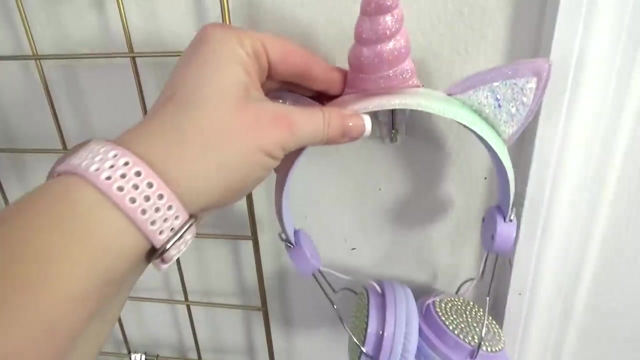 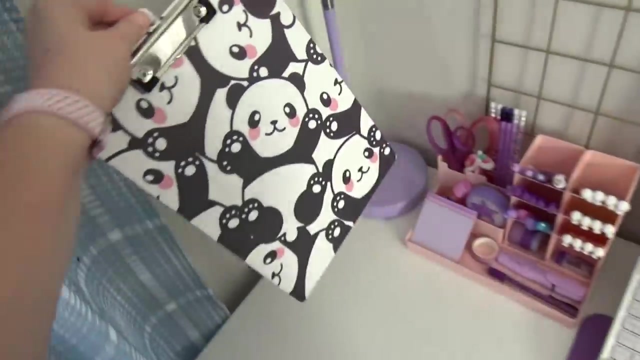 Here we go, And you guys, just like the big kids, Lily also got her own headphones. She has a clipboard for her schedule and her chores. Above her desk, I've left her plenty of space to hang up some new artwork. Art is Lily's favorite subject. 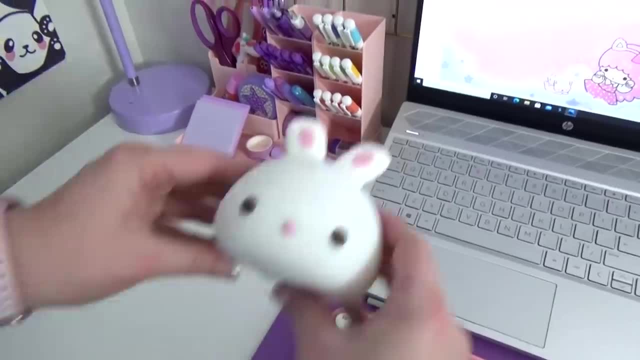 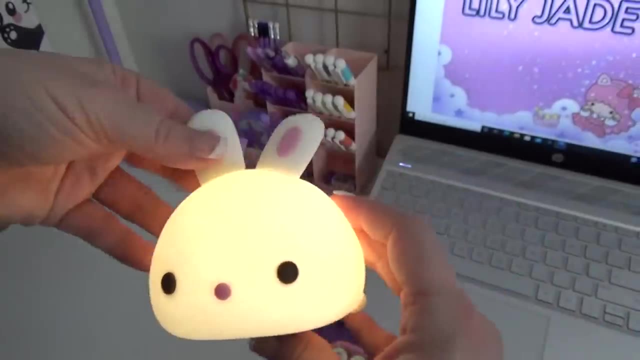 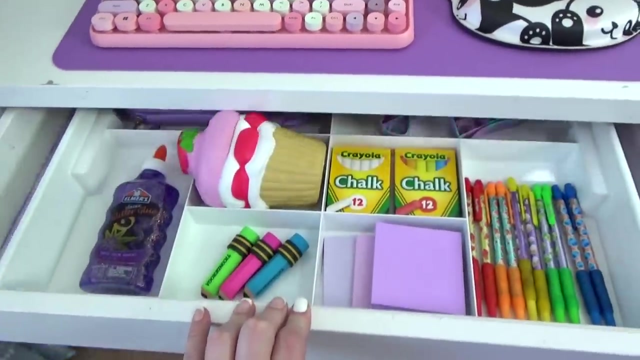 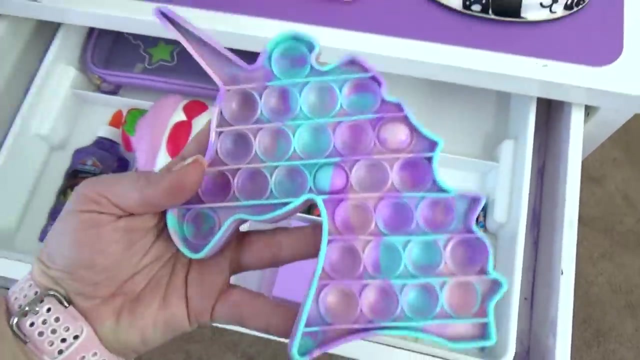 so I know she's going to be making a lot this year, So I'll be reading some of her life stories in the next couple of weeks. I'm excited to get all of those out, and then I'll be reading some of her new books. 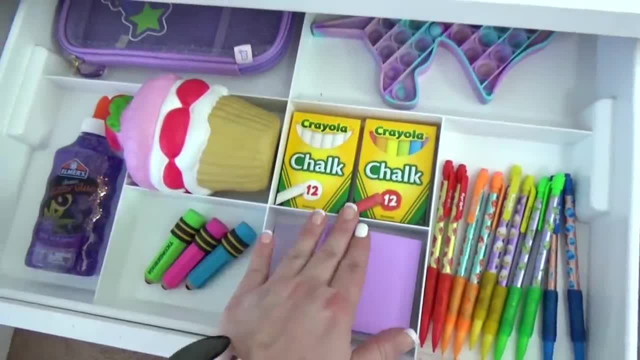 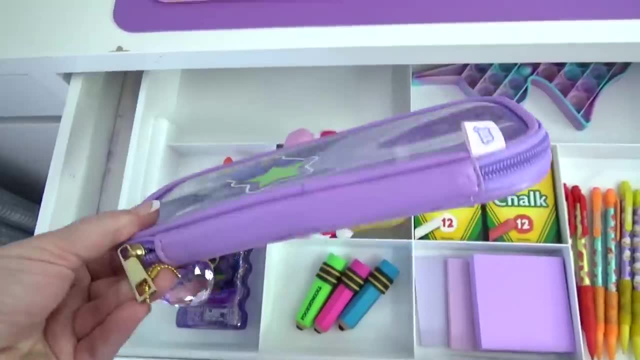 So I'm just gonna sit back here and enjoy the rest And I'm gonna go back to my desk and get some of my stuff laid out. But I'm gonna go ahead and go bring a little bit of my stuff and I'll be right back. 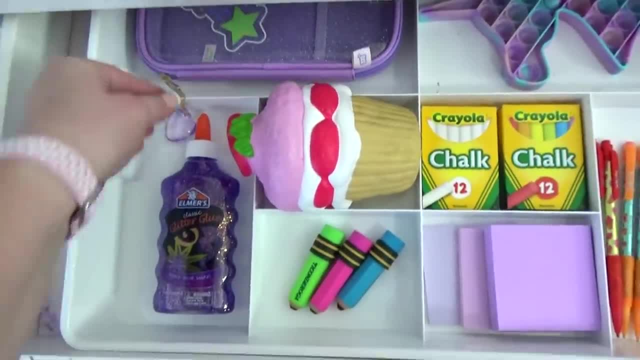 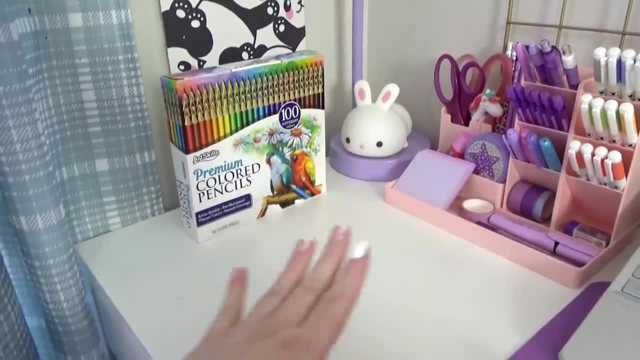 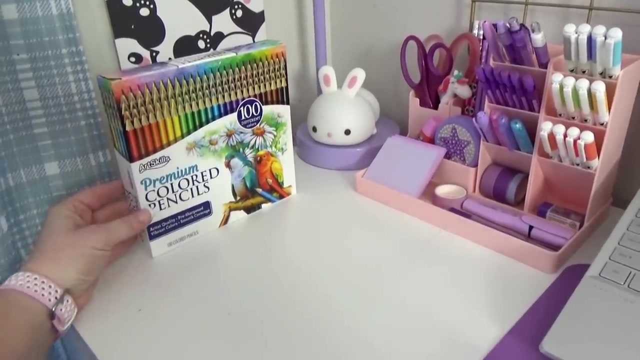 And you guys. speaking of art, one of the things that Lily asked for was a necklace, So I'm gonna show you something: a nicer set of colored pencils. She uses them a lot, so I got her these ones, And I actually ordered a special organizer for these. 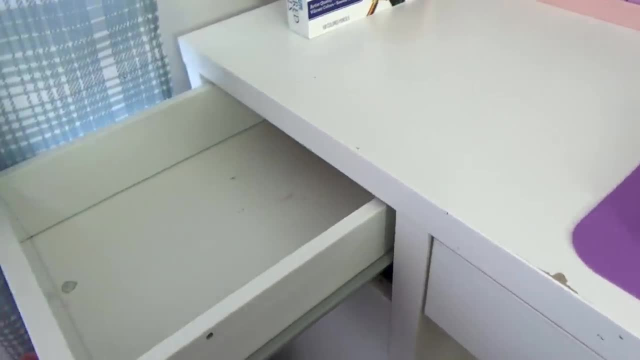 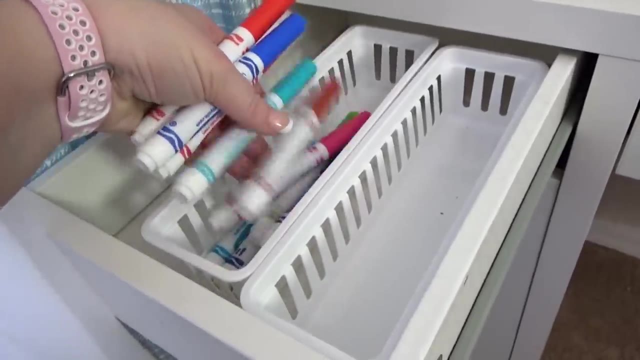 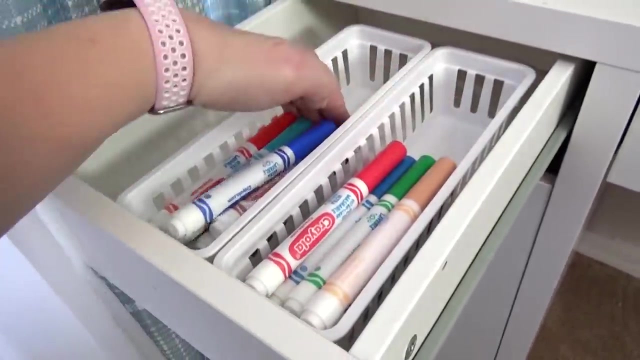 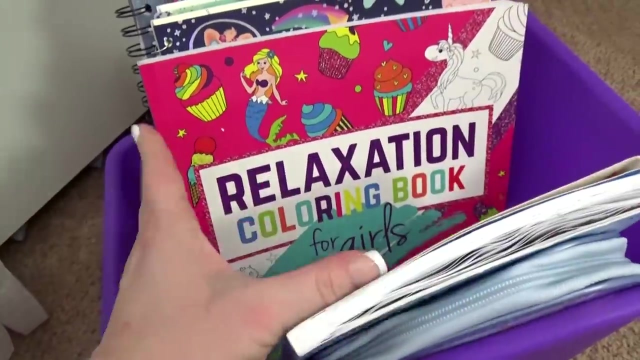 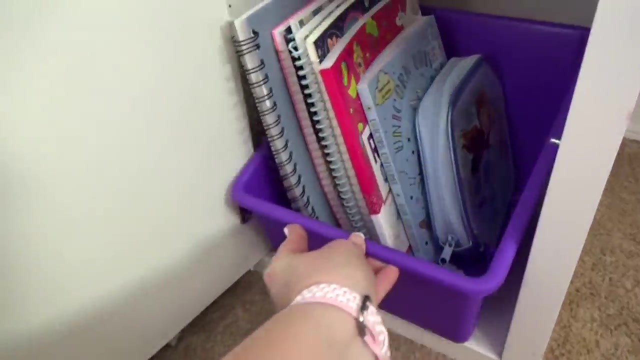 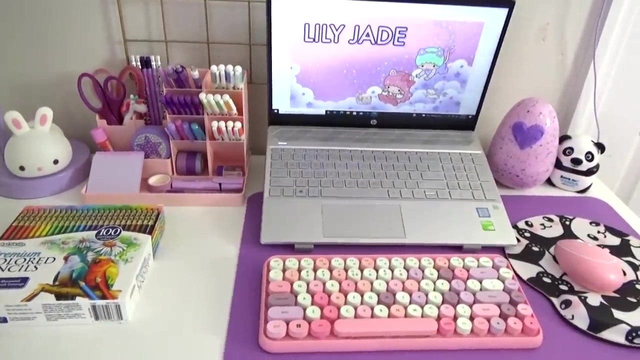 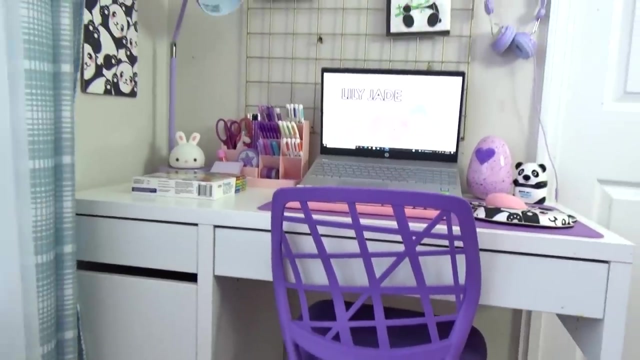 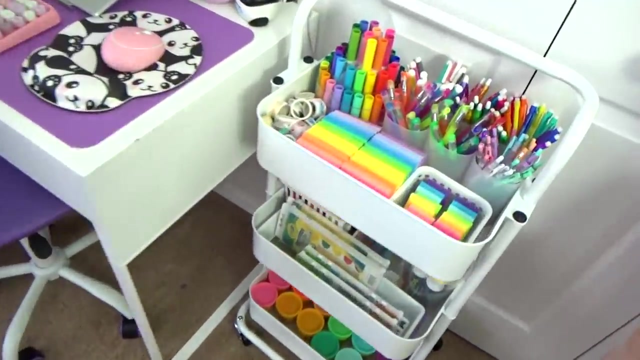 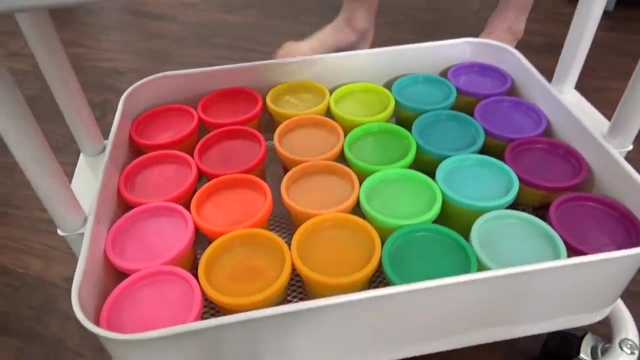 but I'm still waiting for them to come in the mail. Uh-oh, Next to Lily's desk, we're also going to be adding our freshly restocked art cart. Now, this is something that we usually keep in Lily's room, since she uses these items most often. 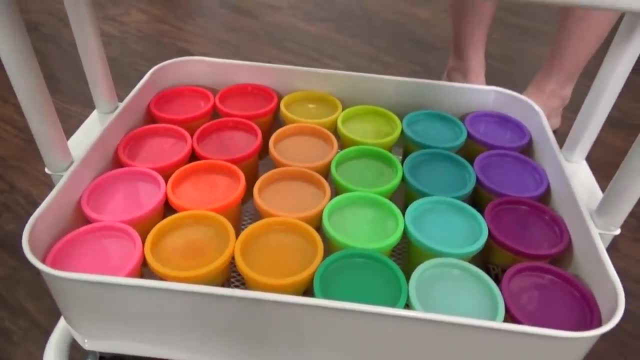 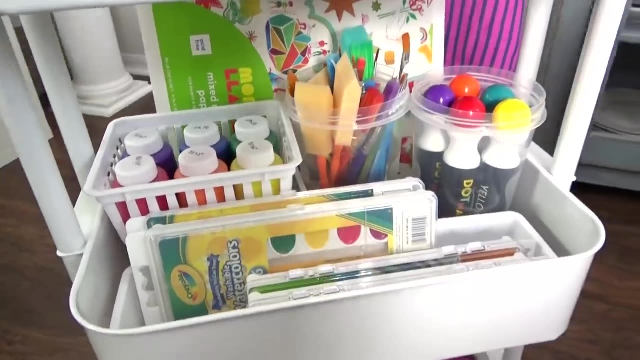 but definitely all of the kids are welcome to use these items. But if we're doing a big art project or we're working on a project altogether, we actually do that at the dining room table, So it's kind of like a second school area. 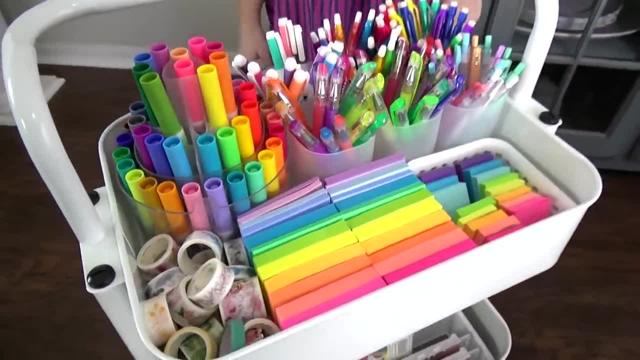 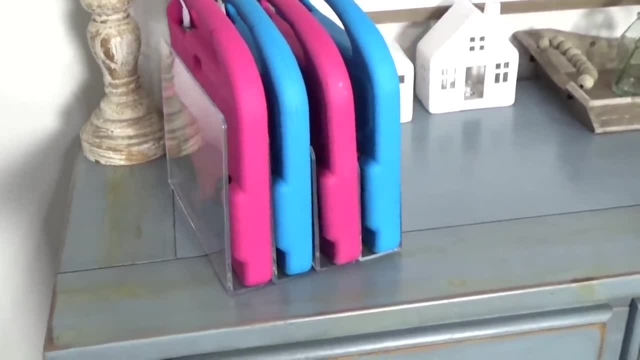 for all of the kids. It's great that this art cart is on wheels so we can easily move it downstairs. In this area we also have our tablet and computer turn-in station. This is where the kids can turn them in when they're done with school. 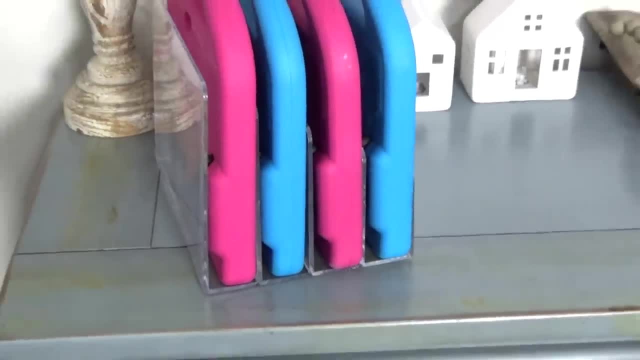 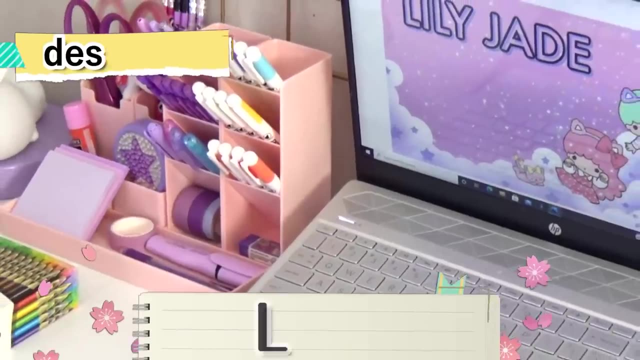 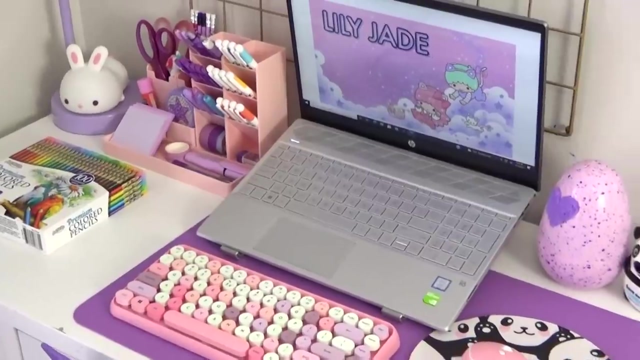 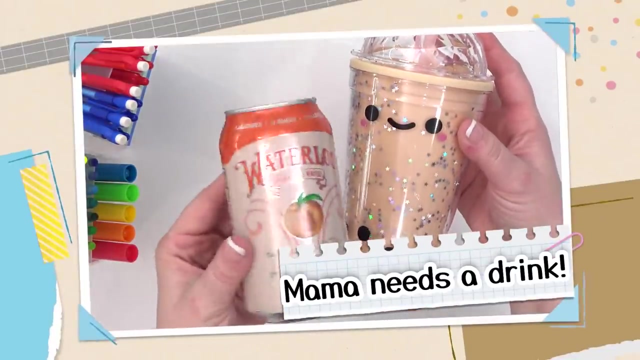 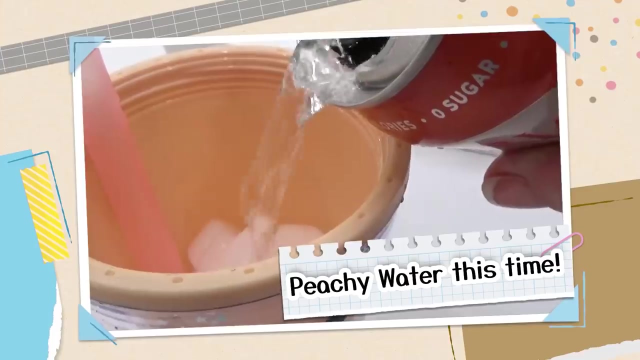 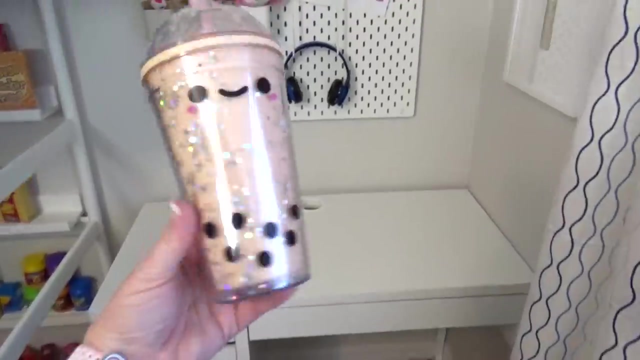 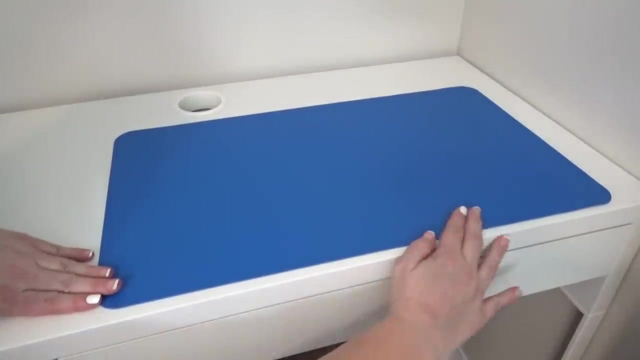 and that way they don't have the computers and tablets in their room all day. Now we just have one more desk to go, but I'm definitely gonna need a refill For Griffin's desk. I got him the blue desk protector. We recently gave Griffin a London-inspired room makeover. 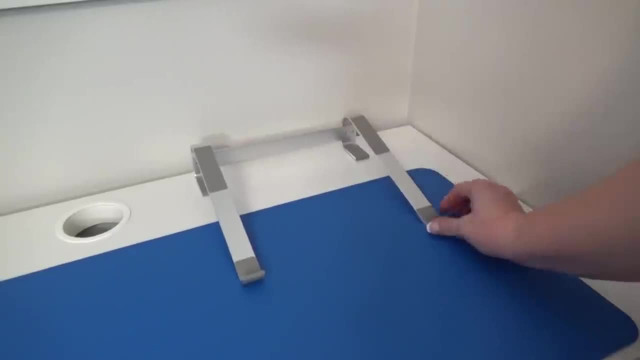 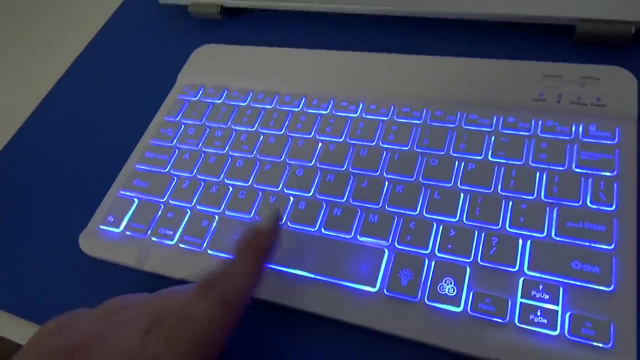 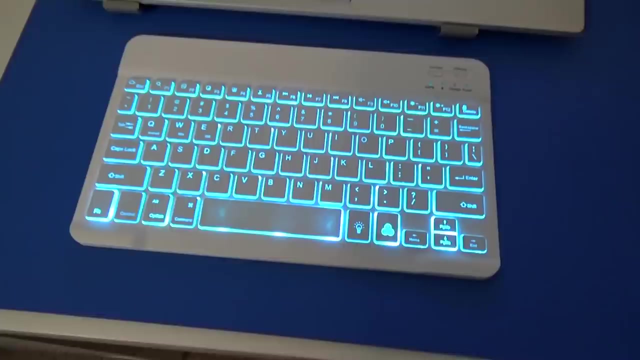 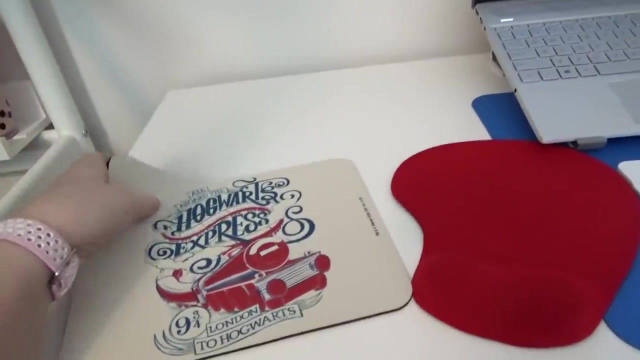 so you're gonna be seeing that theme in the desk area as well. Now, originally I wasn't planning to get Griffin a mouse or a mouse pad, since he doesn't spend as much time on the computer doing schoolwork as the older kids do. 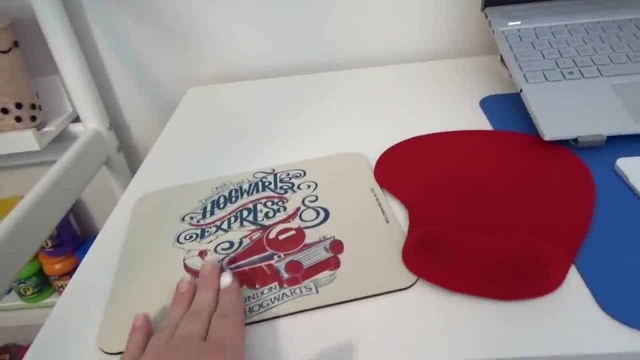 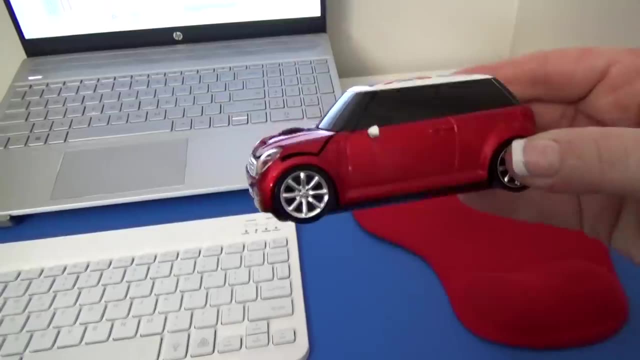 Since I got them for all of the other kids, I decided to get him some too. And you guys? the mouse pad was kind of a hard decision. Would you check out this adorable mouse? It looks exactly like a car. The little headlights even light up. 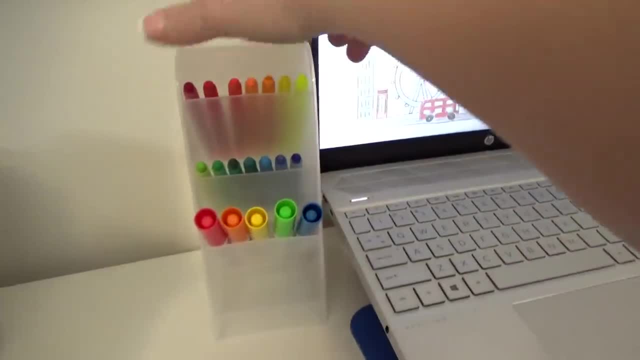 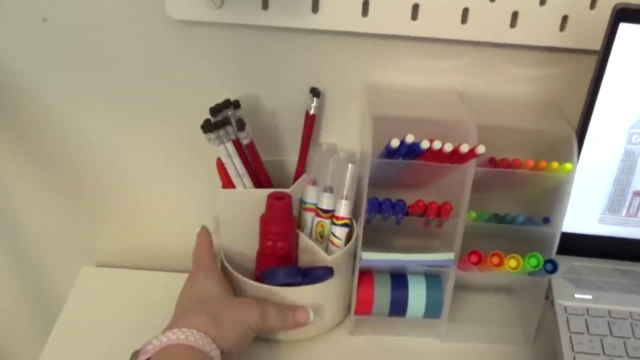 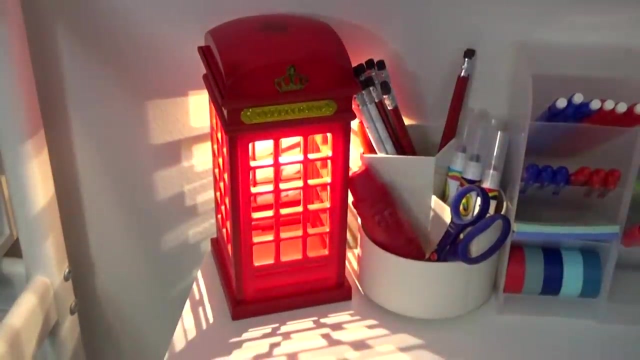 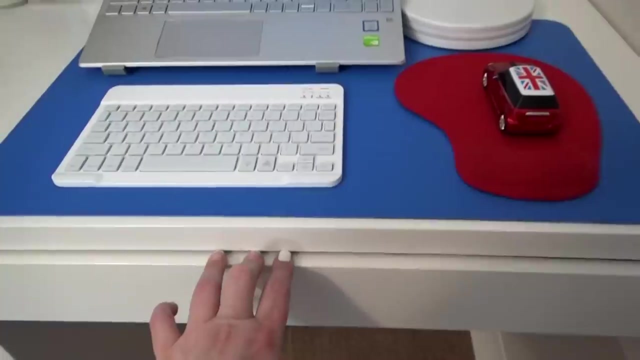 when you click the buttons, But it just makes it look like a computer desktop, And that's a great idea, And I also have a little black desk so I can just leave it there to go. But these are pretty easy to clean up. 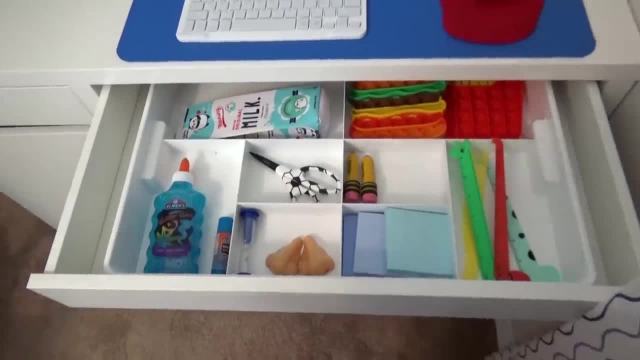 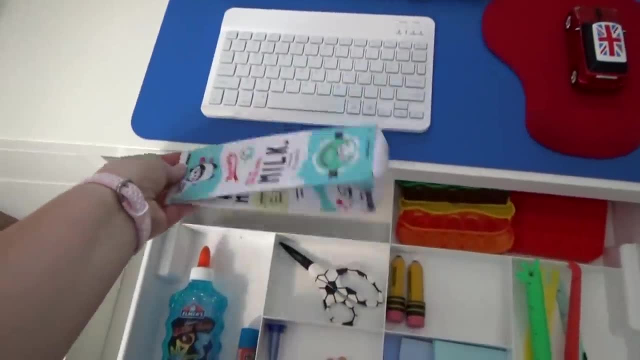 All you need is to clear those iPad Tao buttons and then there's a mouse pad right there and you can just help pick them up every time you're done. So this is my mouse pad And this is my keyboard. Let's see if I can figure out where it goes. 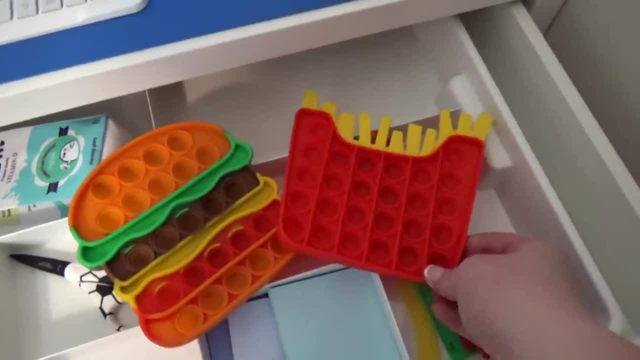 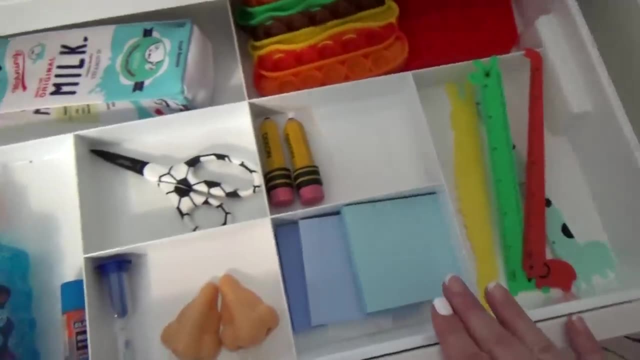 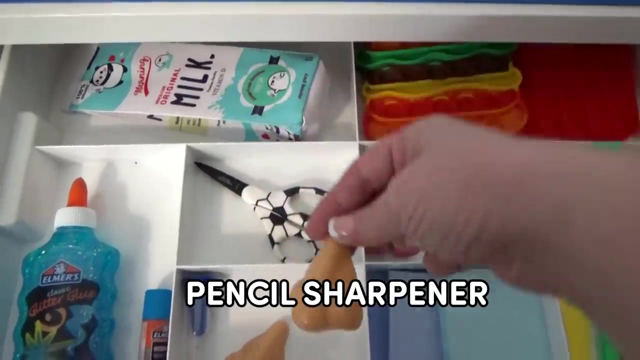 So it has the one icon for as many buttons as possible. Now the mouse pad on this keyboard. let me cut it out. I'm going to use this as a base for the stove. I'm going to use this as a base for the stove.